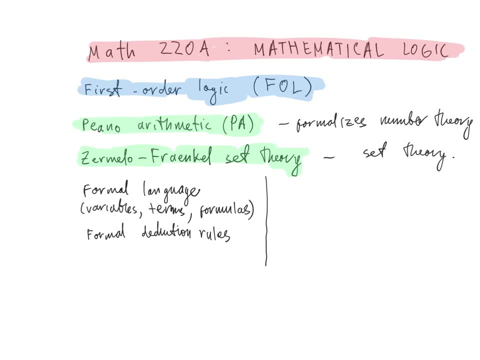 are purely symbolic and no specific interpretation or meaning is given to the symbols, So all of this is syntax. On the other hand, structures, sometimes also called first-order structures for a given language, are sets or models where it is possible to interpret terms and formulas. 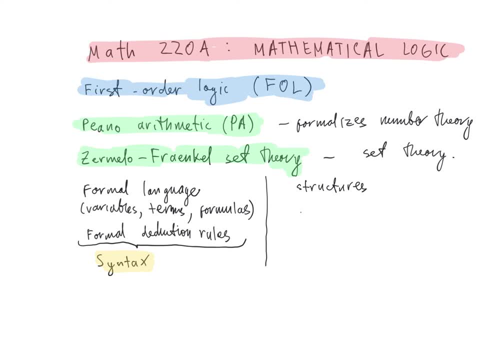 In particular one can give meaning to the validity or satisfaction of a formula in a formal language with no free variables inside a given structure. All of this corresponds to the semantics of first-order logic. 2. någon cents e 3.. 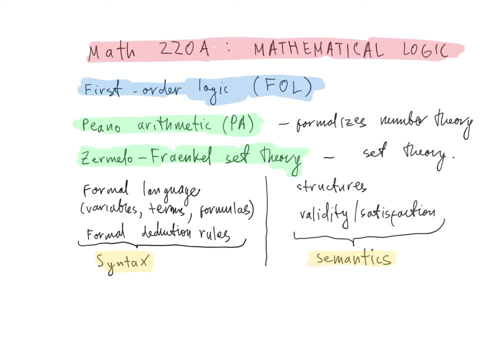 кофейни. The first fundamental result of our course will be Gödel's COMPLETENESS THEOREM, A fundamental result in mathematical logic which states that a formula with no free variables can be formally deduced from a given set of axioms. 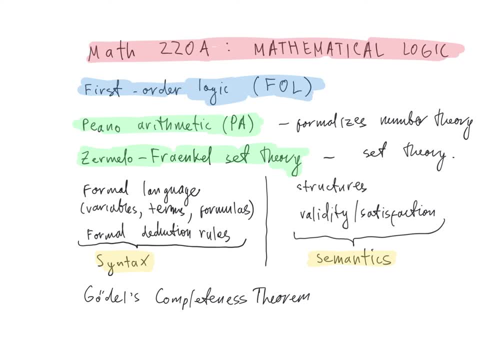 axioms, if, and only if, it is valid in every structure satisfying these axioms. This remarkable result shows that the syntactic and the semantic viewpoints are equivalent. It also provides an a posteriori justification for our choice of syntax, including the semantic rules and the formal language. 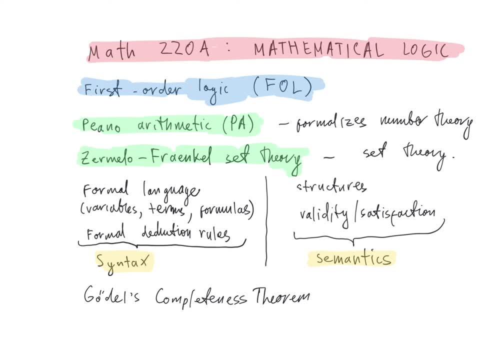 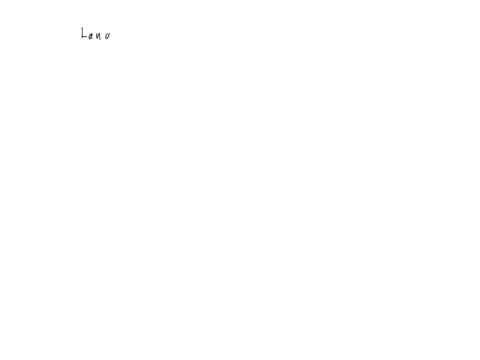 In other words, it shows that there are many possible different choices for these formal rules, but all of them ultimately give the same result. Let's begin by making all of this precise. So we begin with the discussion of languages and structures. Statements in first-order logic are just sequences of symbols describing properties of certain. 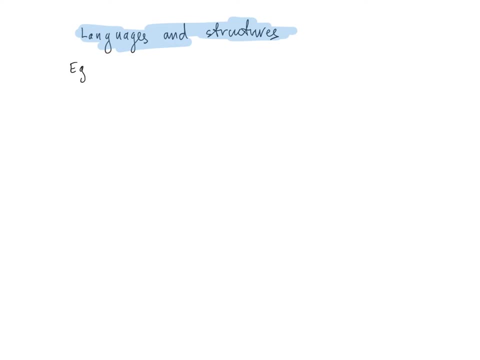 mathematical structures. For example, we can consider the following expression: for all x, x is greater than zero implies exists y, such that y times y is equal to x. Very importantly, this is just a sequence of symbols from a given fixed, finite alphabet. 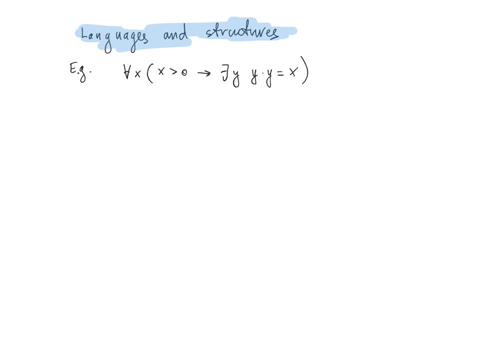 We don't impose any meaning on it by a priori. So in the usual interpretation of these symbols in mathematical practice that we have seen before, this is a sentence which holds in an ordered field. So this sentence holds in an ordered field if, and only if, every positive element is equal. 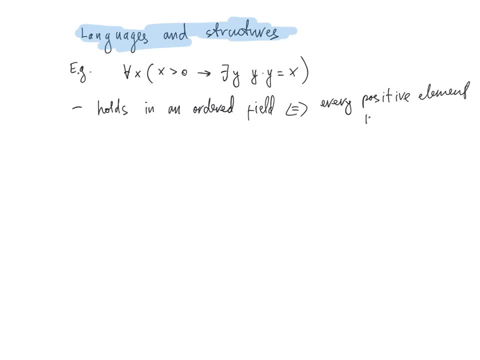 to zero. In particular, note that it holds in the field of real numbers equipped with the constants 0,, 1, the symbols for addition, multiplication times and less than all. interpreted in the usual way we interpret the separations on the real numbers. 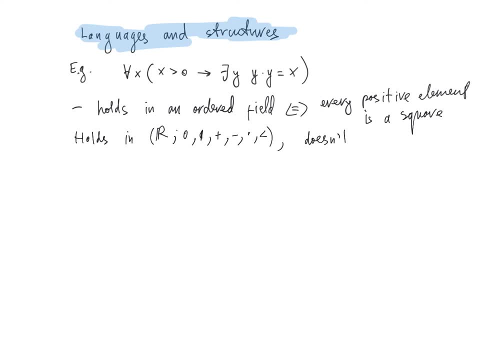 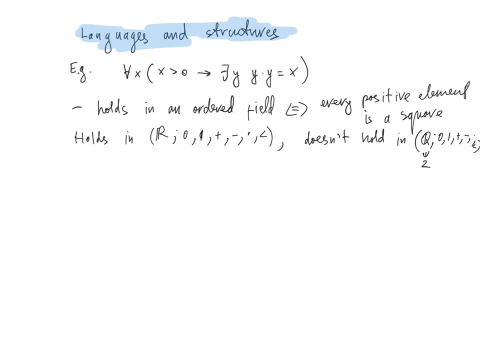 well-known that the square root of two is an irrational number. It is well known. It is well known. It is well known number, so that its square is equal to 2.. We will see that this statement can be expressed in first-order logic. One important point, however, is that some 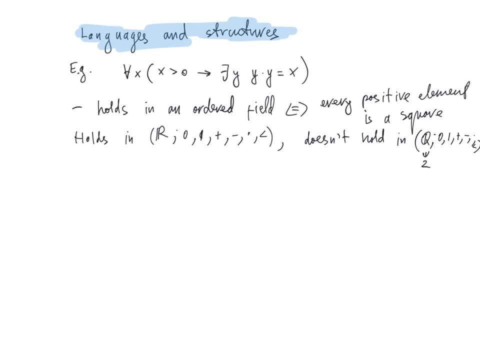 other properties of ordered fields, for example, being complete or Archimedean, etc. cannot possibly be expressed in first-order logic. In order to be able to talk about all of these notions and questions in a rigorous manner, we begin with the definition of a first-order language. 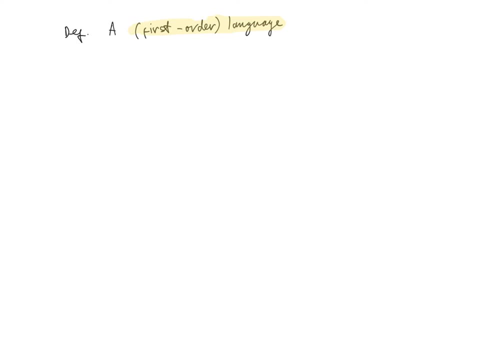 A first-order language, or just language for brevity, is a set of symbols, typically denoted as L, composed of two disjoint subsets. The first part, which will be common to all languages, consists of the auxiliary symbols left bracket and right bracket, together with the 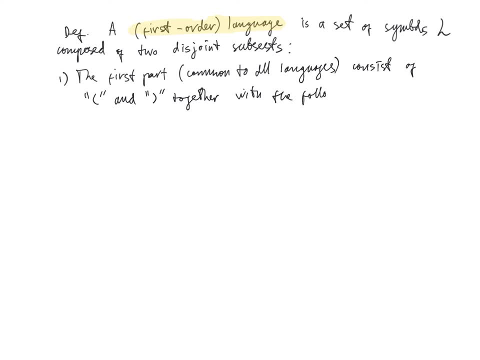 following so-called logical symbols. so, which include the set of variables which will denote as curly v, and it consists of the variables vn, so just elements of the set. vn. for n, an arbitrary natural number, so it's a countable set of variables. It also includes the equality symbol, so just a single symbol equals. 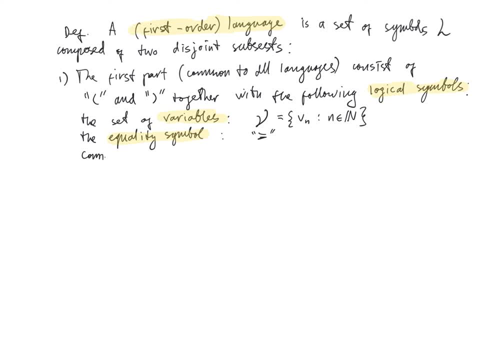 It also contains symbols for the connectives, for which we include the negation or not, and we include the conjunction symbol or and. And finally, we have the existential quantifier, Which is represented by the reflected symbol, capital letter E, and is read as there exists. 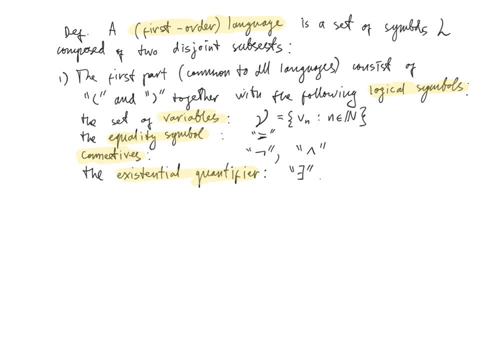 So note that all of these are just elements of some abstract set L. There is no meaning attached to any of them. The second part of the language L, called the signature of L, which is denoted as sigma, superscript L, consists of the so-called non-logical symbols. 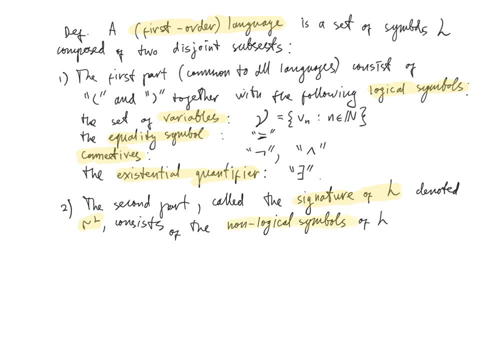 of the language L, And this is the part which is specific to the choice of the language L. It consists of the following: First, a set of constant symbols which will denote as C, L. Second, a sequence of sets- F, N, L. 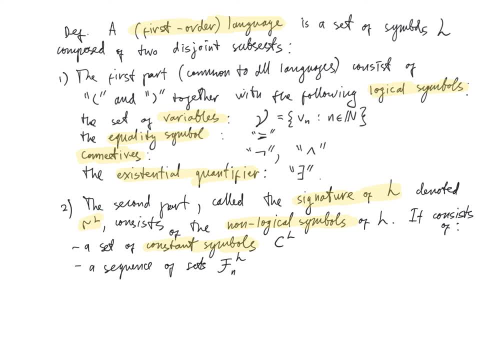 So L still represents that all of them correspond to the language. L and N is a natural number greater or equal than one, where the elements of the set F and L are called the n-ary function symbols. And finally we also have a sequence of sets. 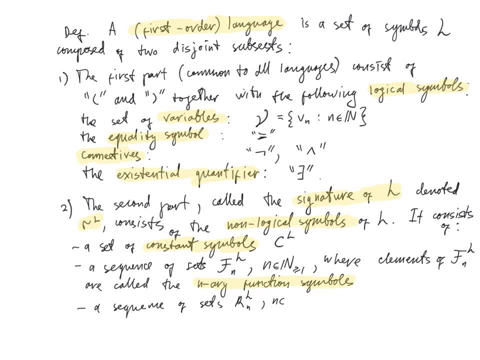 R and L for N, a natural number greater or equal than one, where the elements of R and L are called n-ary relation symbols or n-ary predicates, The language L is given by the disjoint union of these sets of symbols. Let us stress that, while the names of the subsets of the language 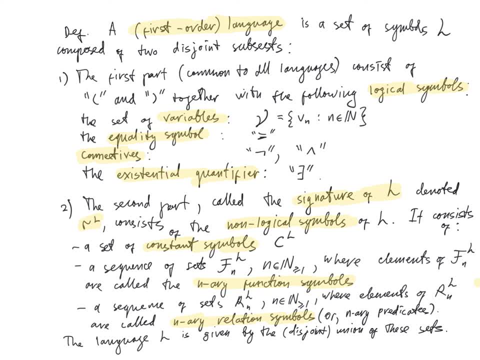 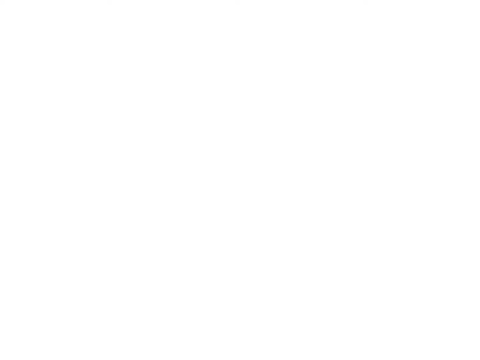 are rather indicative and suggest some possible interpretation. at this point we are not assigning any meaning to them at all. So we just have a set of elements and we subdivide them into several parts corresponding to all of the names listed here. Let us make a couple of remarks. 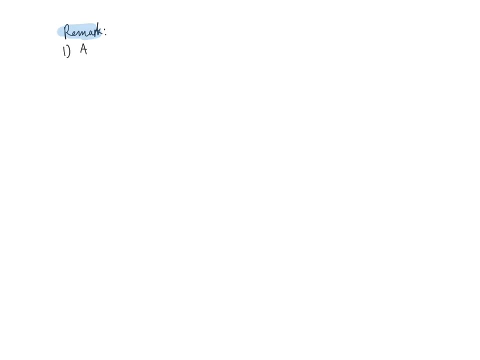 First, a language is always infinite. Note that the logical part of the language is in fact just countable. so the collection of all logical symbols is countable, while there is no restriction on the cardinality of the set of the non-logical symbols of a language. 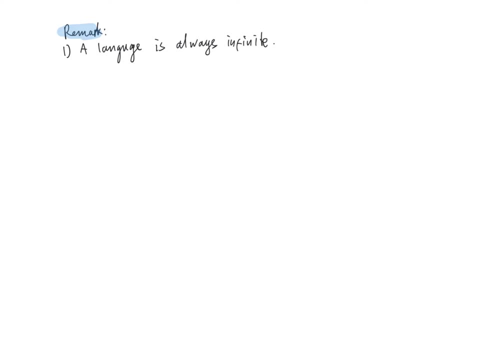 It might be larger than countable. As we already stressed, the first part, the logical part, is common to all possible languages according to our definition, So we might abuse the notation slightly and often identify the whole language L with its non-logical part, sigma L. 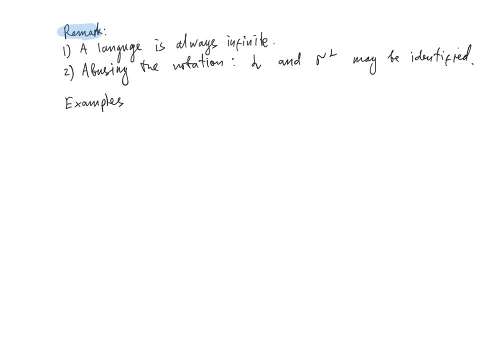 Let's give a couple of examples of languages that we will encounter later on in the course. First, consider the language L empty set, which is not going to contain any symbols at all. So to this we refer as the empty language. Note again that here we are identifying L and sigma L. 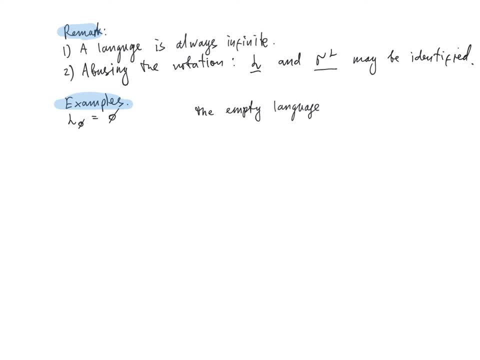 So, of course, L empty set still contains all the logical symbols which are, by definition, included in every language, but it doesn't contain any additional non-logical symbols at all. Next, we will let L ring be the language whose non-logical part consists of the symbols 0 and 1,. 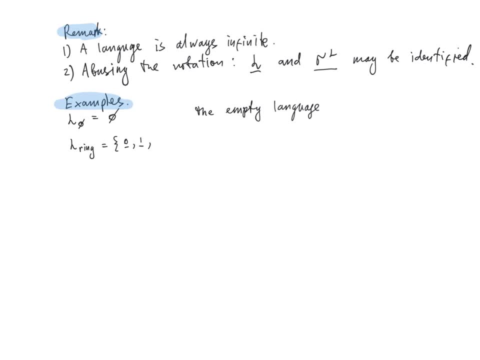 both constant symbols and three binary function symbols denoted as plus, minus and times. We refer to this as the ring language. Another example is given by the language L ord, which consists of a single binary relational symbol less than 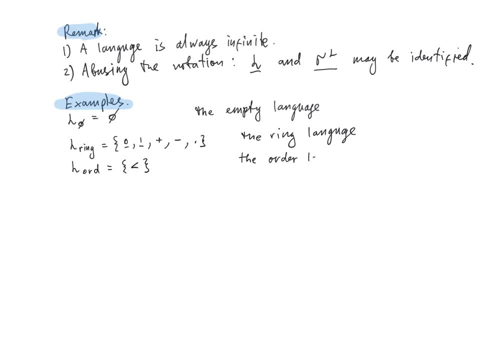 We refer to this as the order language. The next example is the language L ordered rings, which we take to be the union of the language of rings and the language of orders and referred to as the ordered ring language. We can also consider the language L set. 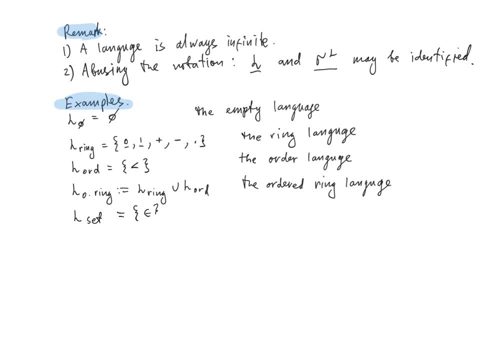 which consists of a single binary relation symbol denoted by the belongs to symbol, and refer to this as the language of set theory. Let's consider one more example. Let L groups denote the language consisting of a single binary function symbol denoted by the times operation. 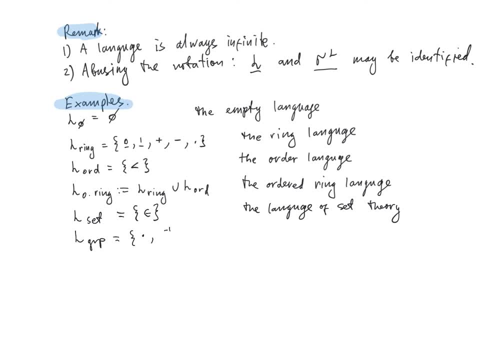 It also contains a single unary operation denoted by the inverse operation, and it contains a single constant: 1.. So this is the language of groups. And finally, one more, the language of graphs, L graphs, which consists of a single binary relational symbol: E. 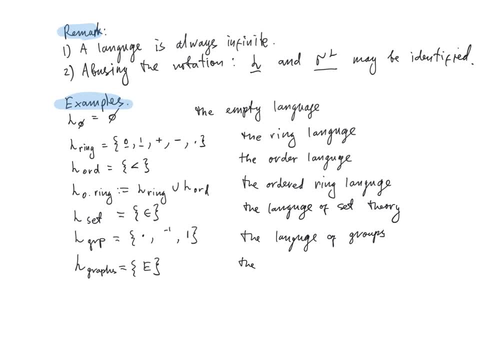 which, in the future, will be used to denote the edge relation. so the language of graphs. And let's consider one more, the final language, the language which we denote as L? R. it consists of a single constant symbol denoted by 0,. 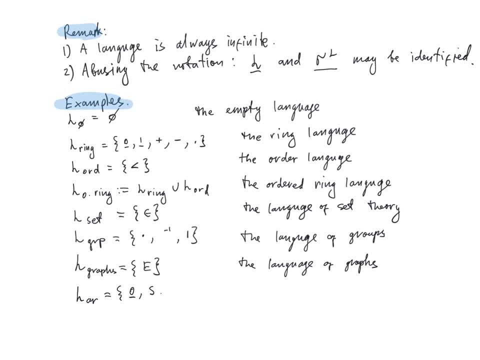 a single unary function symbol, S, a binary function symbol plus a binary function symbol, times, and a binary relation symbol, less than which we will refer to as the language of arithmetic. Let me stress once again that, at this point, all of these are just arbitrary sets of symbols. 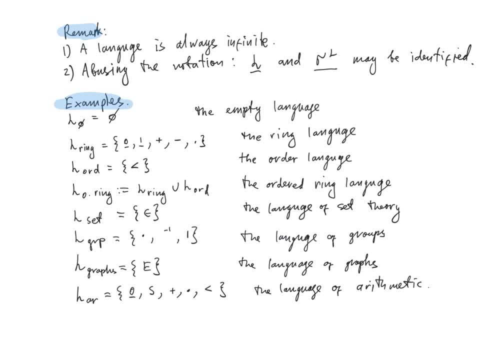 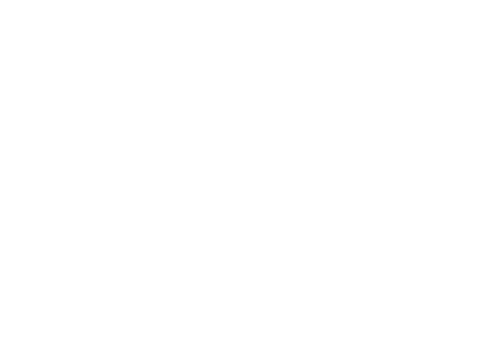 denoted in this particular way, but there is no meaning attached to them, no interpretation is attached to them, And our next definition will allow us to start connecting these symbols with the intended meaning for them. Definition: Let L be a first-order language. 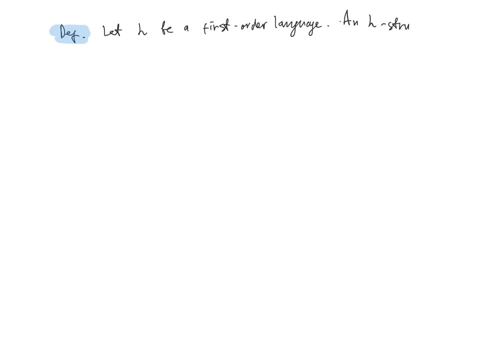 an L structure a consists of a non-empty set A, called the base set of the structure A, together with an element C A in the base set A for each constant symbol C of the language. L, a, function, F, subscript, curly A. 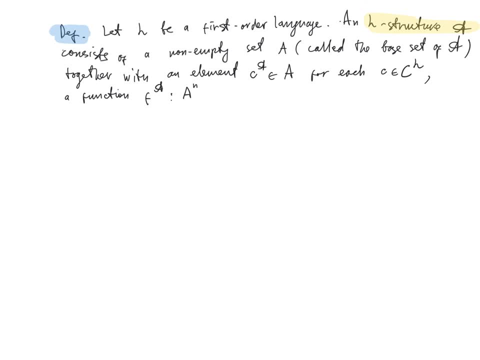 from the base set A to the power N to the base set A for each function, symbol F of arity N from the language L and a subset R, curly A of the N's power of A, the base set. 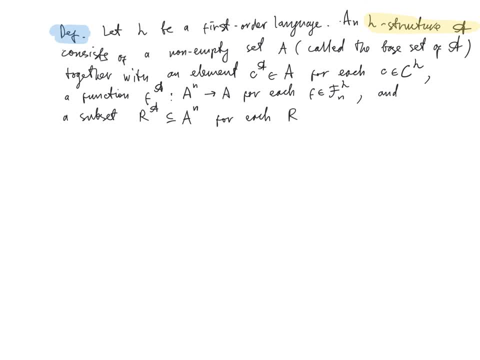 for each relational symbol R from the language L of arity N. Given such an L structure, we will write that the structure curly A consists of the underlying set, A, the base set, and it consists of the symbols Z, capital, A. 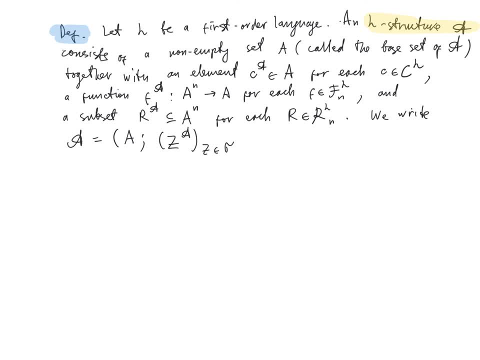 where Z is a non-logical symbol of the language L, Now the object Z, subscript curly A, which can be either an element of the base set, a function from some power of the base set to the base set. 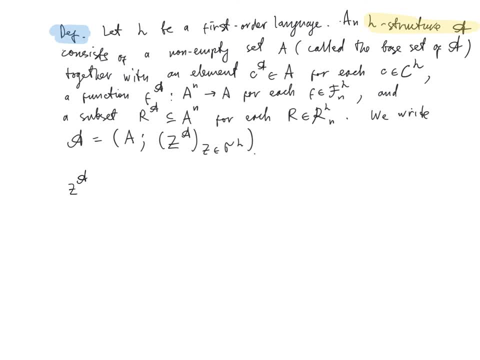 or a subset of some power, of some finite power, of the base set. A is called the interpretation of this symbol. Z in the set of all non-logical symbols of the language. L in the structure. 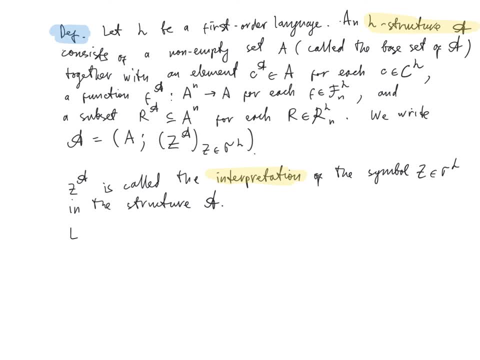 curly A. Let us consider some examples of structures. Example one: consider the structure curly N to be a structure in the language of arithmetic. the base set, the set of all natural numbers, the constant symbol zero. 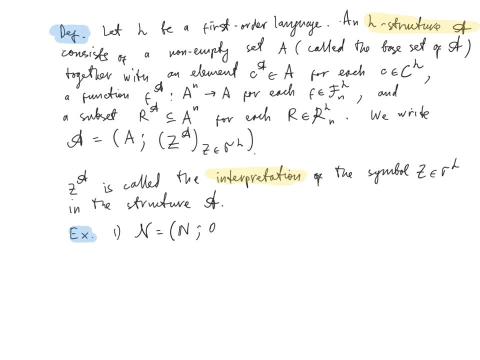 interpreted as the actual number zero in this base set. the function symbol S, the unary function symbol, interpreted as X, goes to X plus one. a function, the successor function from the base set to itself. 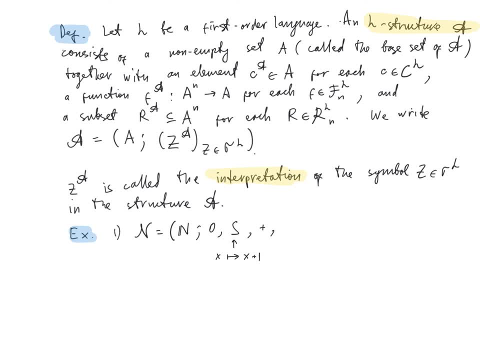 and the remaining function symbols: plus times, interpreted as the usual addition and multiplication on the set of natural numbers. and finally, the ordering, interpreted as the usual order on the natural numbers. so, together with all of these, 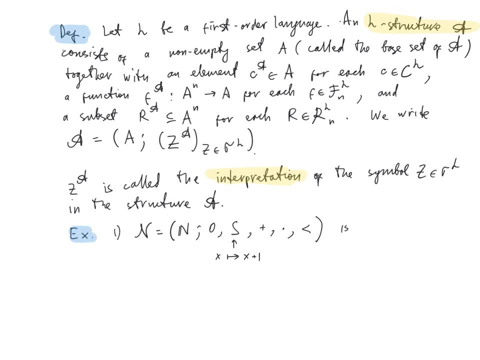 interpretations. curly N is an L R AR structure, a structure in the language of arithmetic defined previously as the set of complex numbers and the interpretation of the constant symbols by zero and one. 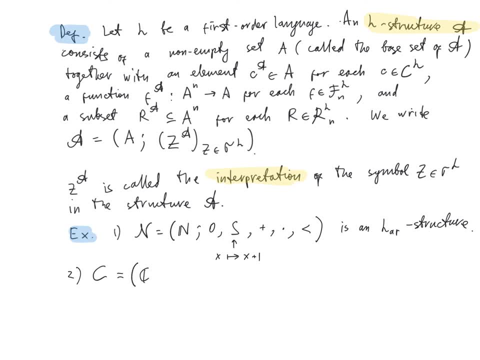 the actual complex numbers zero and one and plus minus and times, all interpreted as the usual additional addition, subtraction and multiplication on the set of N and plus minus and times, all interpreted as: 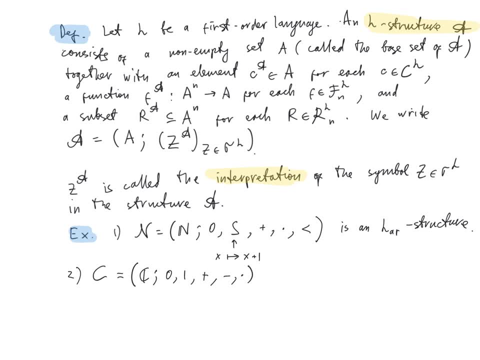 the usual addition, subtraction and multiplication in the set of on the in the field of complex numbers. so with all these interpretations, C is a structure in the language L-ring of rings. and let's consider one more example. 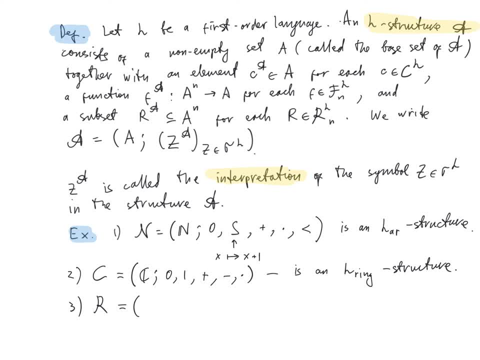 which we'll denote as curly R. so now this is a structure where the ordered rings consisting of the real numbers are: and zero, one plus minus times less than all, interpreted as the standard. 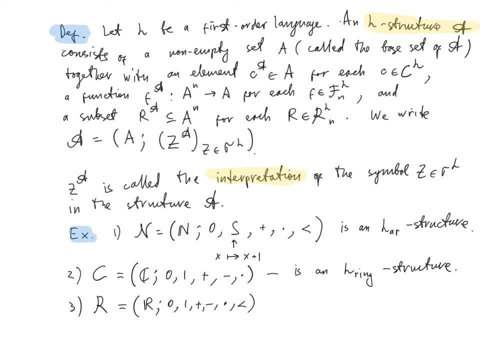 functions, the standard operations in the field of real numbers, the ordered field of real numbers which, with these interpretations, is a structure in the language of ordered rings, having defined L-structures for an arbitrary language. 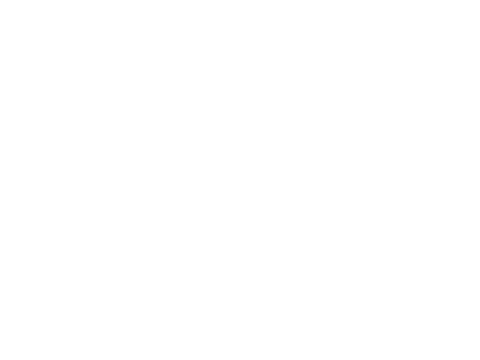 L. we will also now define the corresponding notion of isomorphism of two L-structures in the same language, generalizing the various familiar notions of isomorphisms from algebra, for example. 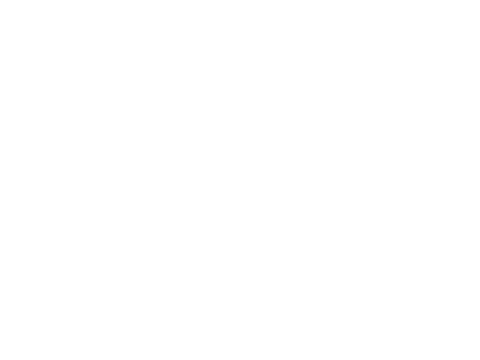 isomorphisms of groups, rings, fields, etc. as well as some notions from combinatorics, such as the isomorphism of graphs or hypergraphs. so we have definition. we will say: 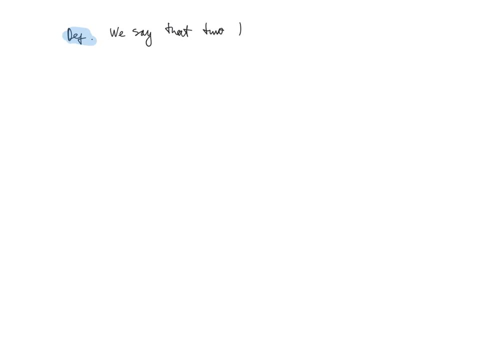 that two L-structures, A and B, are isomorphic, denoted symbolically as A is isomorphic to B, if there exists an isomorphism F between A and B. 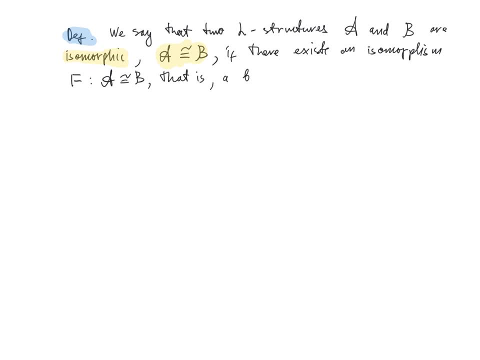 that is a bijection F from the base set of A to the base set of the L-structure B. so a bijection between the base sets A of curly A and 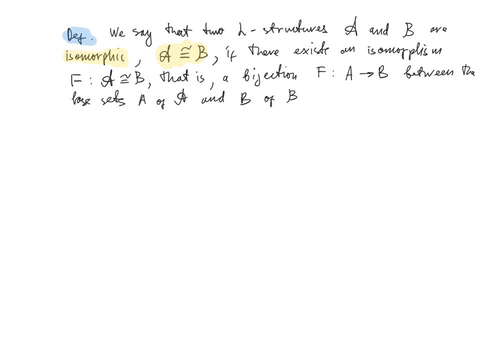 the base, set B of the L-structure, curly B, which commutes with the interpretations of the symbols in the signature of L, in the non-logic part of L. so what do we mean by commutes? 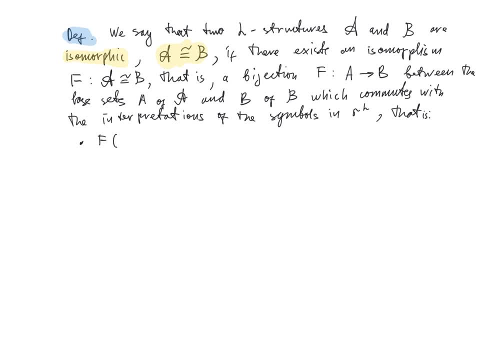 that is first. we have that F. the function capital F applied to the interpretation of the constant symbol C in the structure A sends it to the interpretation of the same constant symbol C. 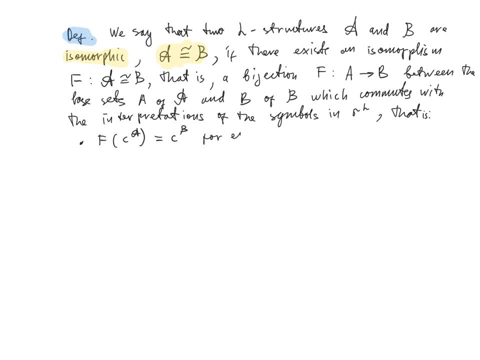 in the structure B, and this holds for every constant symbol C among the constants of the language L. secondly, we have that the function capital F sends, let's say, composed. 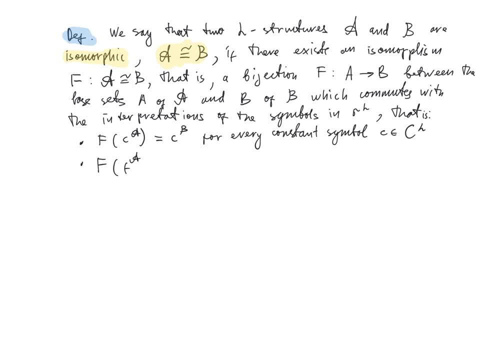 with the interpretation of the function symbol F in the structure: A applied to a tuple A1,, An is equal to F. B applied to the images of the elements of this tuple. 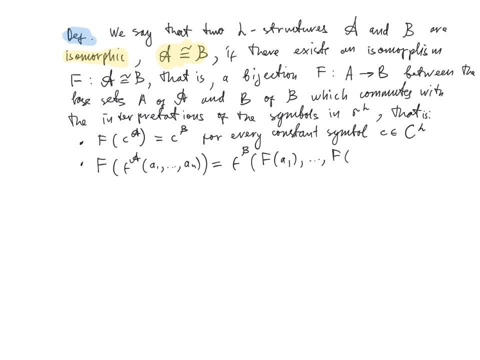 with respect to the function, to the isomorphism, capital F, and this equality holds for every function symbol, little f of arity N in L. that's why we're considering tuples of length. 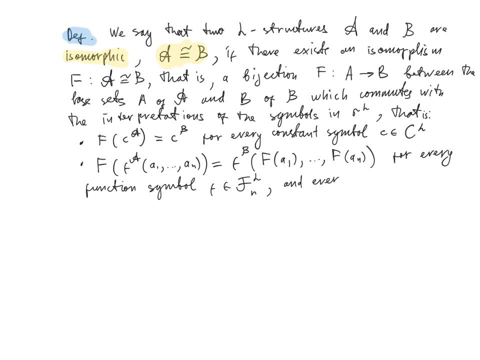 N and every tuple A1, An so of length N in the base set of the structure A, and finally we have that a tuple A1, through An belongs. 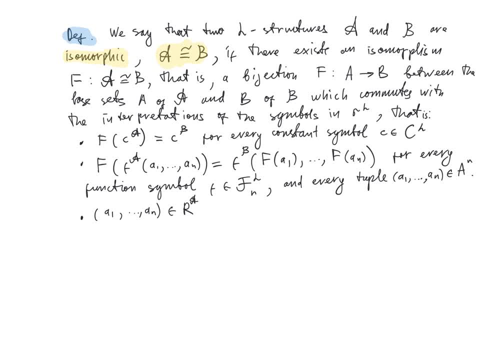 to the set given by the interpretation of R in the structure A if, and only if, the corresponding tuple obtained by applying the isomorphism capital F, so the tuple F of A1,. 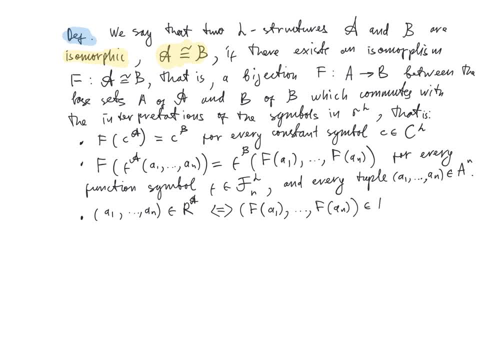 through F of An belongs to R B, the interpretation of the same relation, symbol R in the structure B, and we require that this holds holds for every predicate of R. 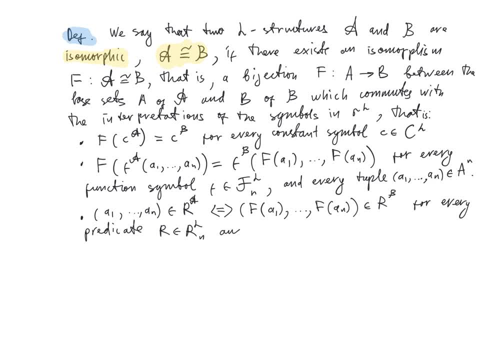 T, N in L and every tuple A1, through An from the base set A of the structure, curly A. similarly, the function F is not necessarily by ejection but satisfies. 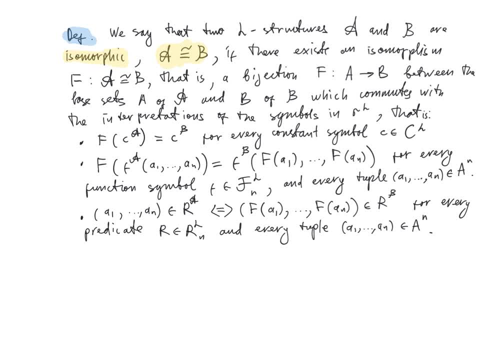 all of these conditions we can talk about F morphism from A to B, and if it is an injection, we talk about an embedding of a structure A into the structure B. 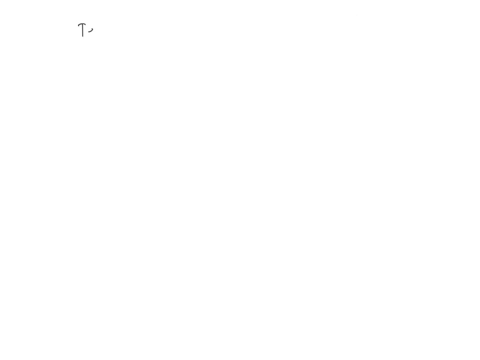 having defined languages and structures, let us proceed to defining related syntactic objects that can be formed given a language, namely terms and formulas. definition: a word over a set or 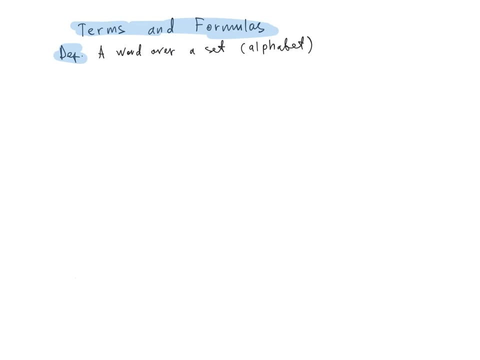 over an alphabet and the current way to refer to this particular set, so that we are considering words. so a word E is just a finite string: A0,, A1,, etcetera A. 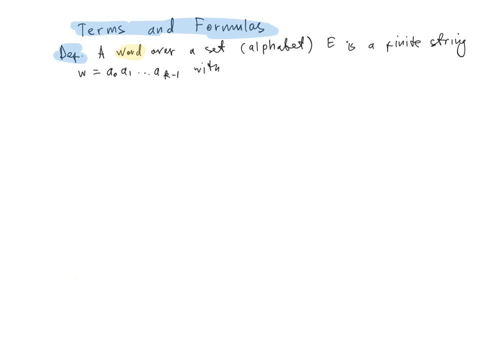 K-1, of symbols from the set E, so with AI in E for every I given such a word, we call K the length of the word W and we denote by: 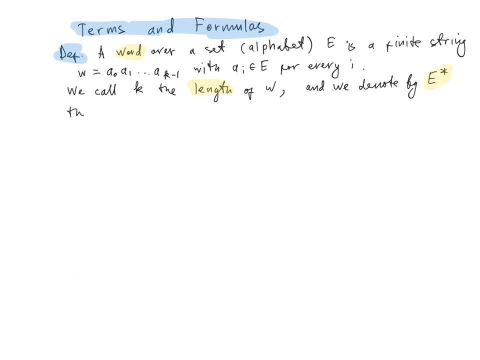 E star, the set of all words over the given set E or the given alphabet E. now we define the L terms of a given language, L, so let L be a language. 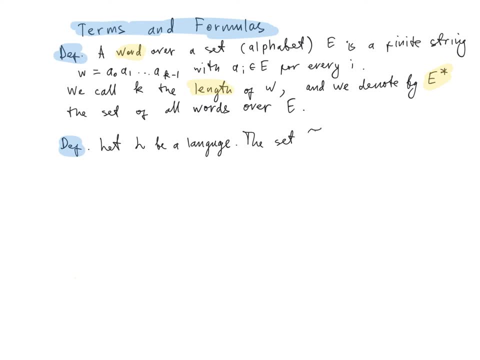 then the set TL of L terms is the smallest subset D of L star. so this collection of all words in the alphabet given by the set elements of the language containing 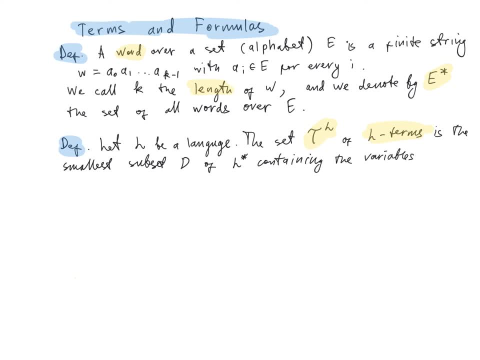 the variables of L and the constants of L and such that if we have a function symbol F of R, T, N from L and we have terms T1, TN in D. 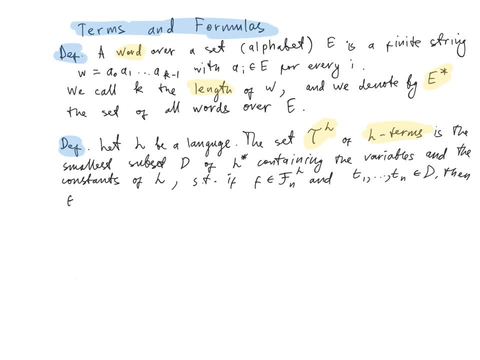 then the term given by the word F, the symbol F, followed by the word corresponding to the term, T1, et cetera, followed by the word for TN, is an element. 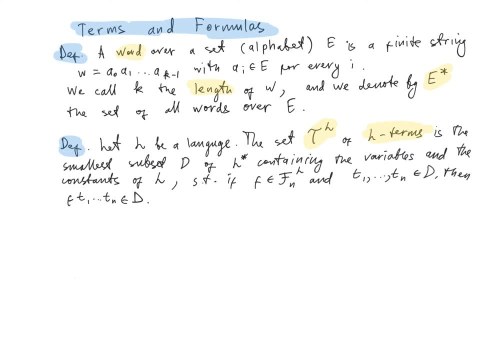 of D as well. here the smallest means the smallest in the set in the sense of inclusion of subsets. this definition gives us a recursive definition for the set of terms, so certain particular. 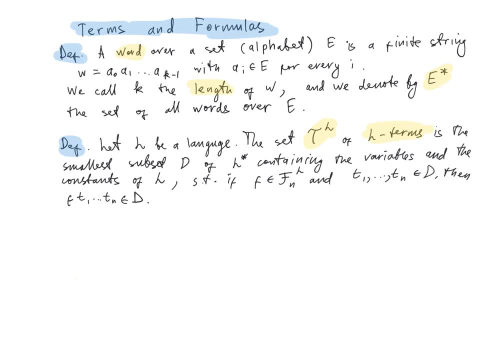 set of words in the language L. so we can use this definition to represent the set as follows: so we can write T: L as the union, countable union over all natural numbers. 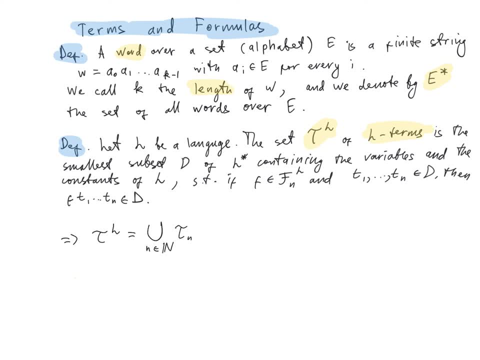 N of T N L, where we have T zero L. so we define T zero L to be the union of the constants, of the constant symbols of the language L. 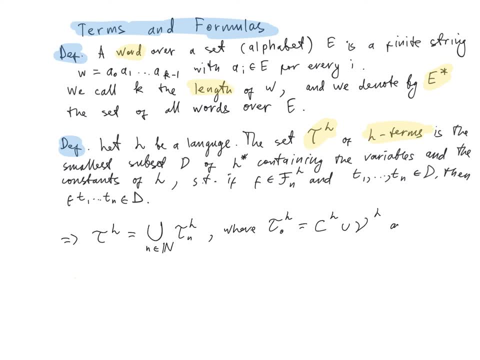 and the variables of the language L, and then, inductively, we have T N plus one L equal to T N L. so all the terms that were obtained. 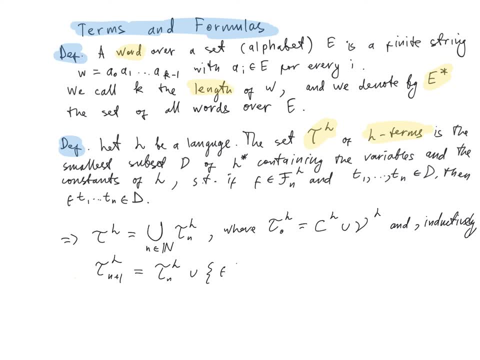 on the previous step, together with all terms of the form F, T, one, T, K. where K is a natural number greater or equal than one, F is a function symbol from. 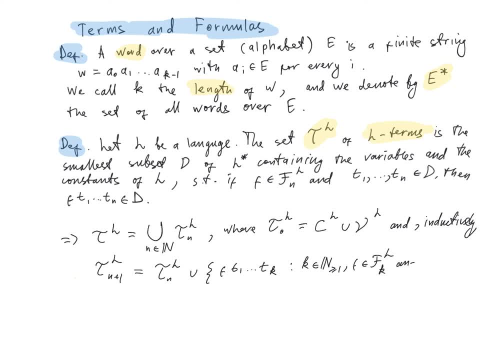 L of R, T K and T one through T K are all terms from the previous level of the construction, so they all belong to T N L. the following: 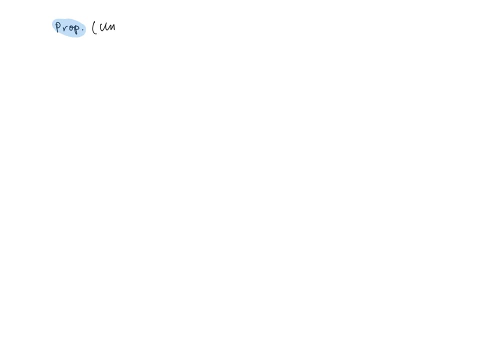 proposition guarantees that term unique readability in the following sense: any term T in a language L satisfies one and only one of the following: the first possibility is that the term T 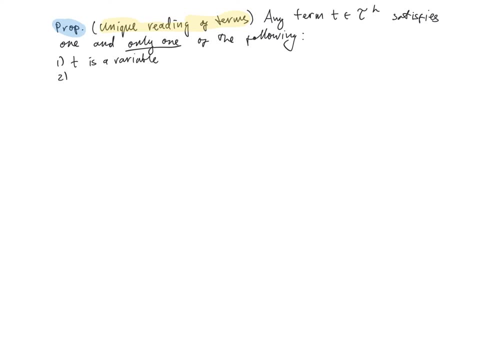 is a variable. the second possibility is that T is a constant symbol and the third possibility is that there exists a unique integer N greater or equal than one, a unique N-ary. 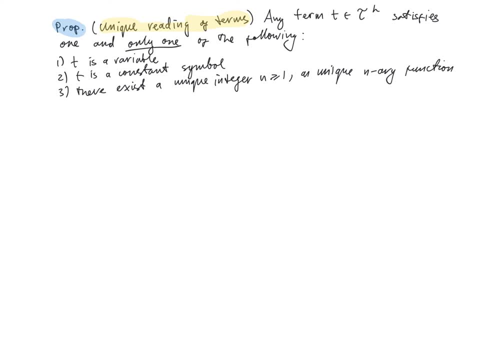 function symbol F in L and a unique sequence, T1, through TN of L terms such that T is of the form F, concatenation T1,, etc. concatenation TN. 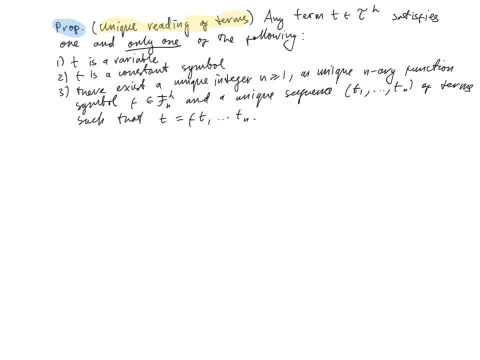 so this is satisfies exactly one of these three options. we leave the proof of this proposition as an exercise. the strategy is to prove first by induction. on the length of terms. 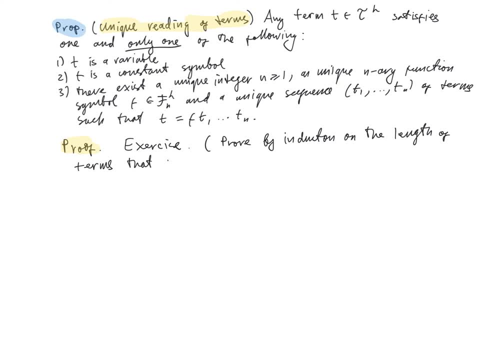 that no proper initial segment of a term is a term. we introduce some notation in order to make it easier to read expressions involving terms. from now on, we shall often write F. 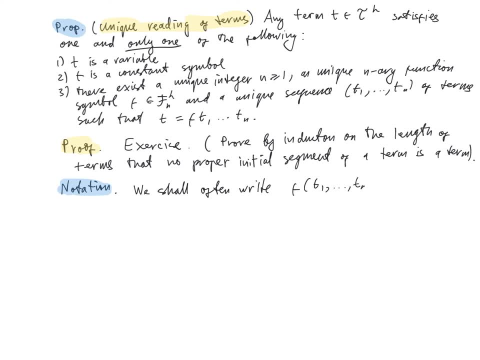 of T1, TN instead of F. concatenation T1, etc. concatenation TN. later we will see that this notation is suggestive and consistent with how terms will be interpreted. 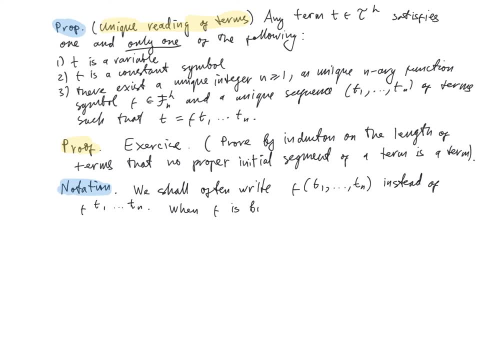 in particular when F is binary. we might also sometimes write T1, F, T2, instead of to denote the term which formally was defined as the term F- T1,. 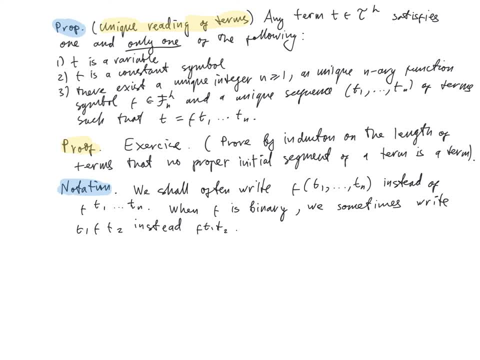 T2,. this is in order to make things more consistent with the usual mathematical notation. so, for example, we can write: X plus Y times Z. this means in the formal definition of terms: 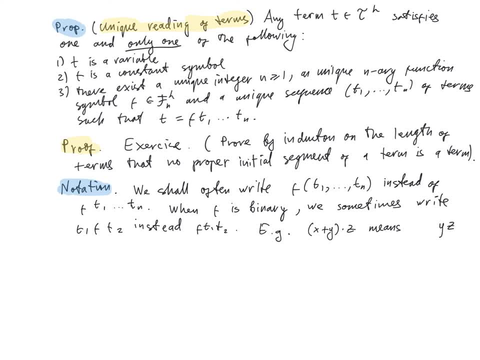 that we made originally. this corresponds to the term Z, Y, X plus times. now the height of a term, T, denoted as HT of T, is defined as the least. 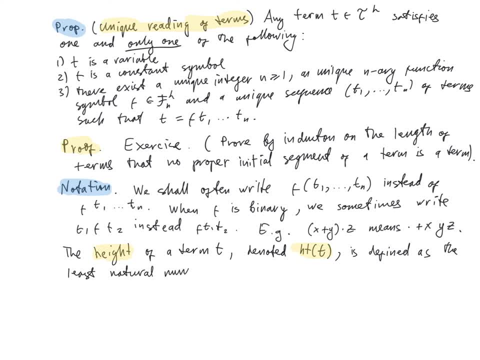 natural number K, such that T belongs to the set T, L, K, so it can be obtained from the constants and the variables in K steps using the inductive procedure that we described earlier. 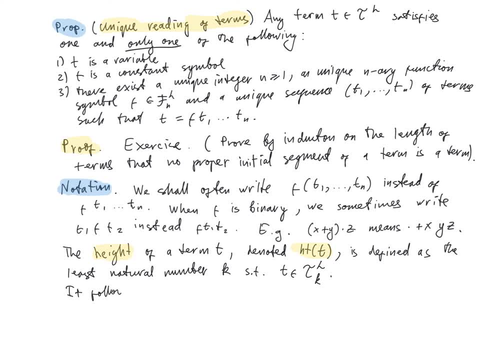 it then follows from the unique reading property for terms, the proposition above, that the height of the term F of T1, et cetera, Tn is just one plus the maximum height. 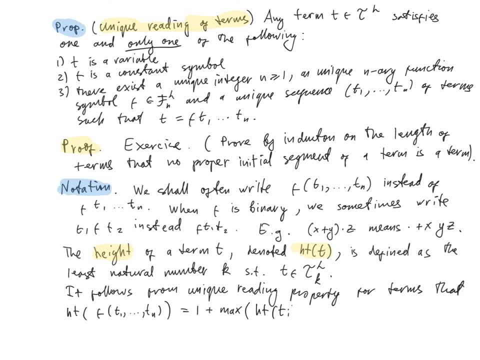 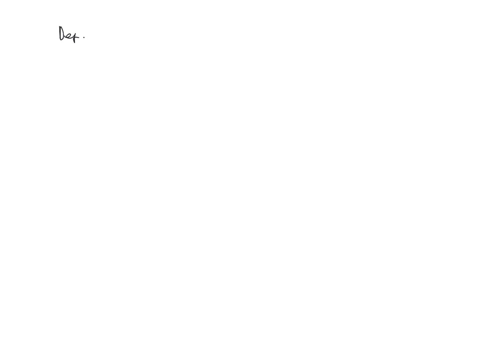 of the terms Ti that appear in it. this simple observation will allow us to give definitions by induction on the height of terms in the future, for the expression of the force over the short form. 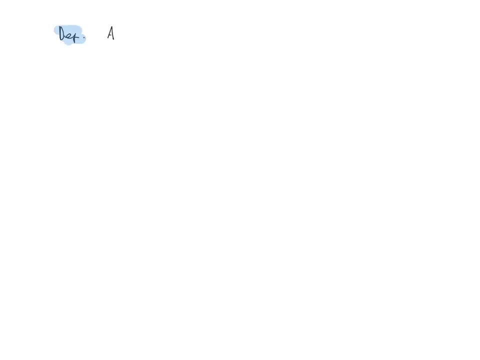 or on the spacer of the term, of the term and in the course of the half of the term or of the term where the force of the invents is the same: plus plus, minus. 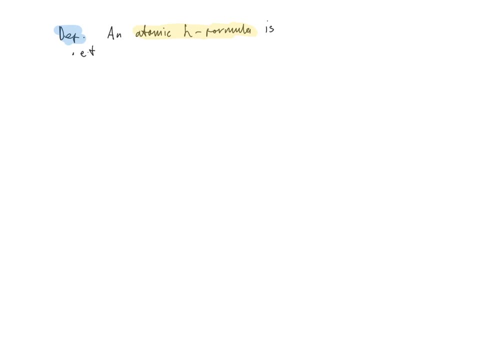 minus, minus, minus, plus, minus, minus, minus, minus, minus. T1 is equal to T2,, where T1 and T2 are L terms or it is a word of the form, R concatenated with T1, concatenated with Tn, where R is a relational symbol of R, Tn from L and all. 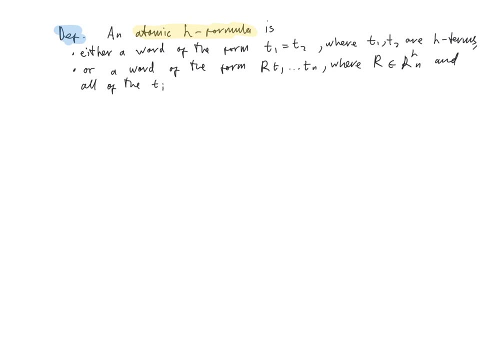 of the Ti are arbitrary L terms. So this defines the set of the atomical formulas And then the set which we denote as FML. L of L formulas is defined to be the smallest, under inclusion subset D Of L star, ie the set of all words in the alphabet on the symbols of the language that. 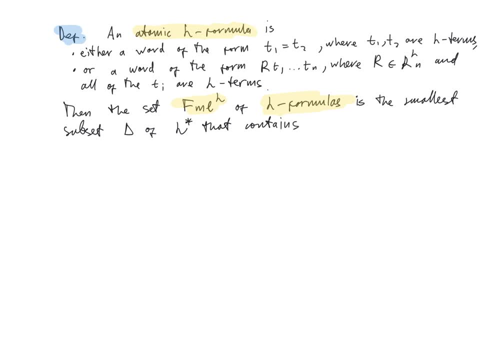 contains all atomic formulas and such that if X is a variable of the language and the set of terms phi and psi are already in D, Then also the words negation, symbol concatenated to phi, the word bracket, phi conjunction, psi, bracket. 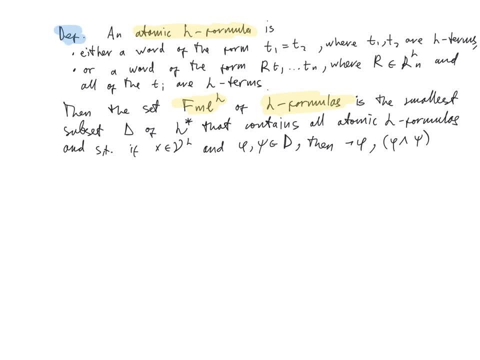 Remember, brackets are the logical symbols in the language- left and right brackets- And also the word existential quantifier of the set of all variables. The word is not phi and the symbol of the language is left and right brackets. Also, it is not a variable of phi and that is why we get Y as phi. 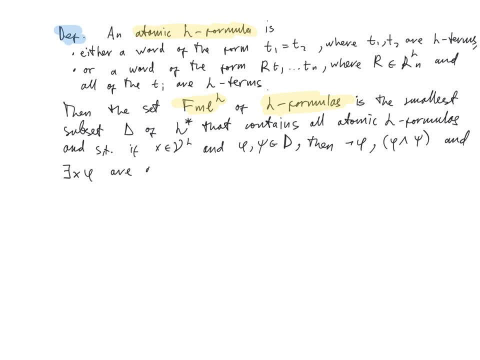 are all in D. This tells us that the new formulas can be formed from the old formulas using one of these three methods. Using this definition, we see that, in fact, the set of all formulas FML in a given language, L, can be written as a union over all natural numbers: N of the sets FML, L, subscript N, where. 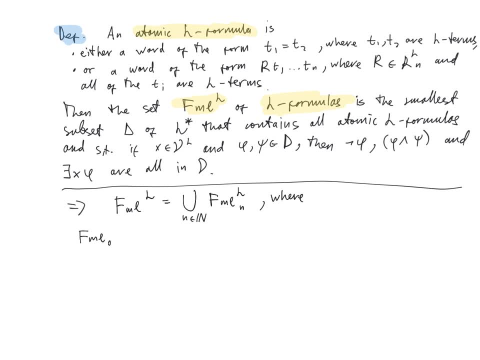 we take FML 0 to be the set of all atomic formulas And we define inductively the set FML L N plus 1 to be the set FML N union, the following sets of formulas: So first we have all formulas of the book. 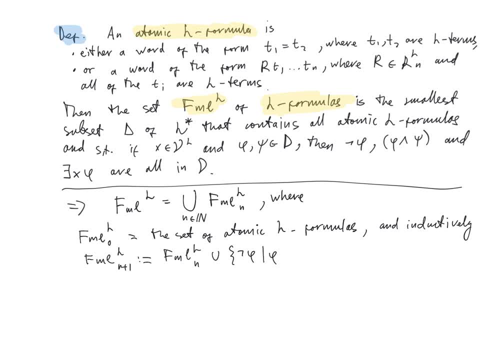 We have the form not-phi where phi is an element of the set obtained on the previous step: FML N, union. all formulas of the form phi concatenation psi. where phi and psi belong to FML N And union, the set exists X. 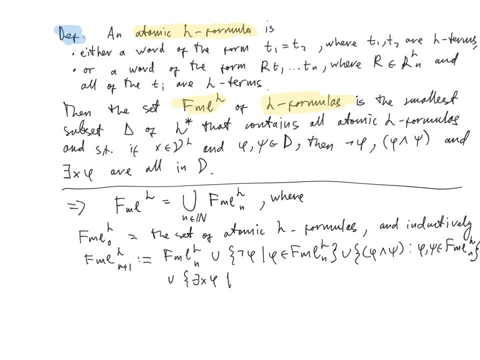 Phi, so that X is a variable of the language, L or just a variable- we don't have to stress the language- and phi is a formula obtained on the step N. Again, the equivalence of these two presentations as the smallest set in the definition and.